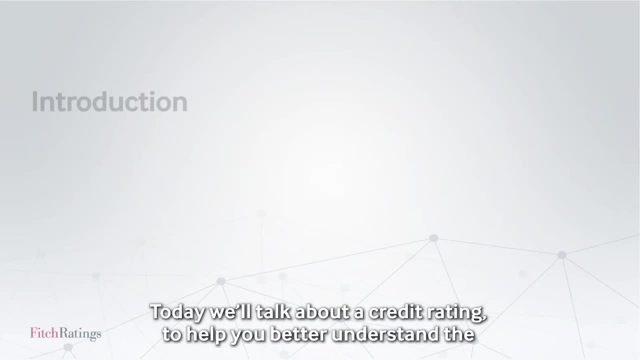 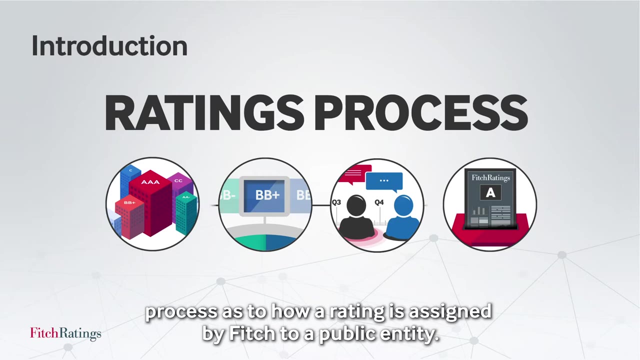 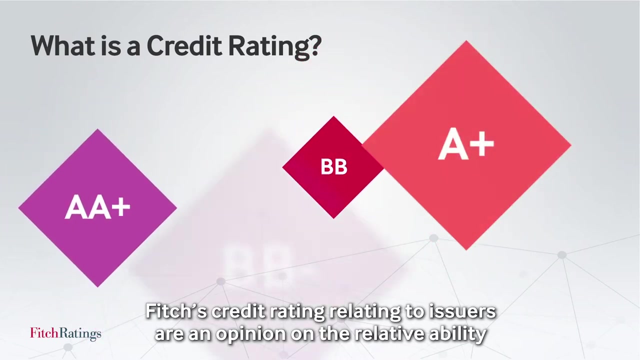 Today we'll talk about a credit rating to help you better understand the process as to how a rating is assigned by Fitch to a public entity. What is a credit rating? Fitch's credit ratings relating to issuers are an opinion on the relative ability of an entity to meet financial commitments. 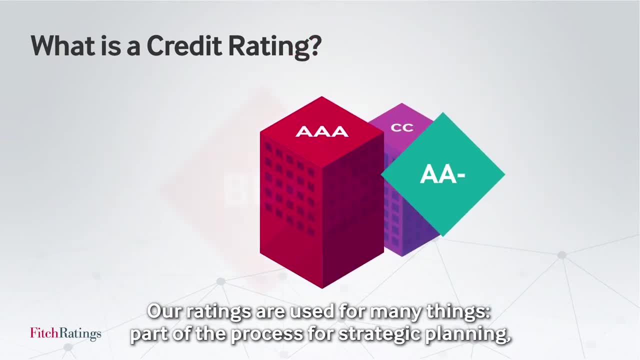 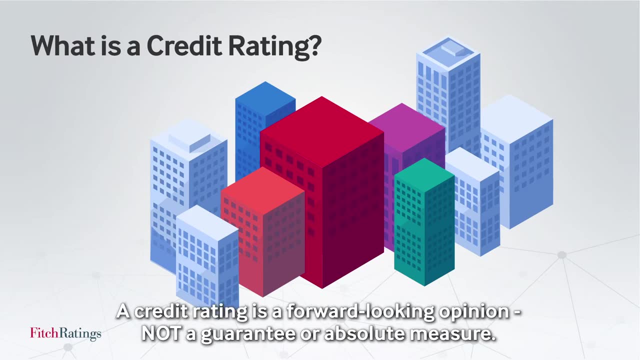 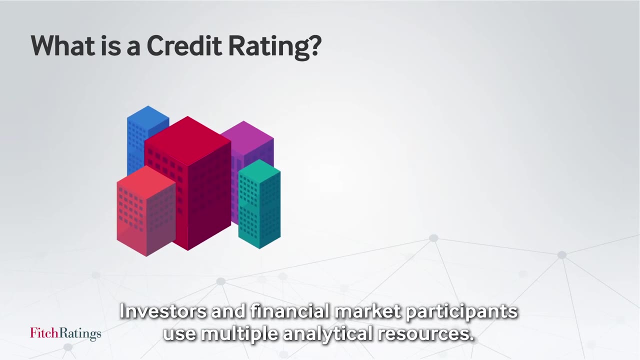 Our ratings are used for many things: part of the process for strategic planning, peer benchmarking and borrowing, lending and investing decisions. A credit rating is a forward-looking opinion, not a guarantee or absolute measure. Investors and financial market participants use multiple. 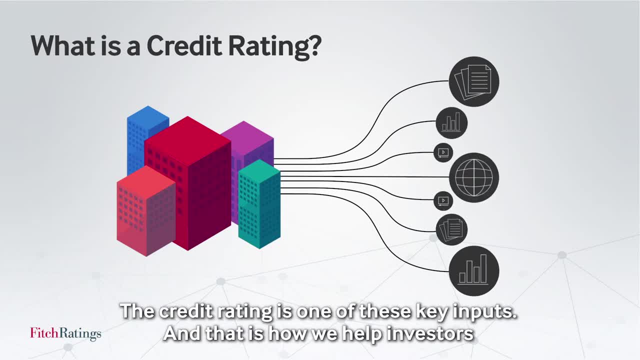 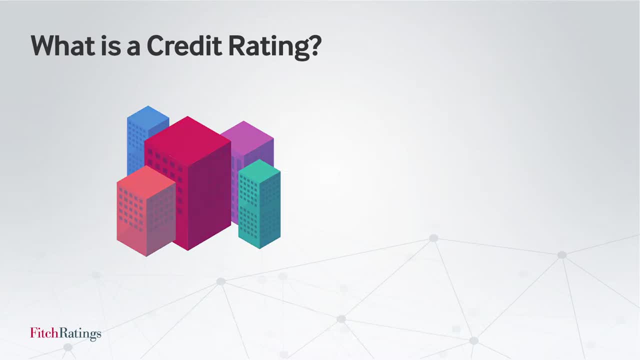 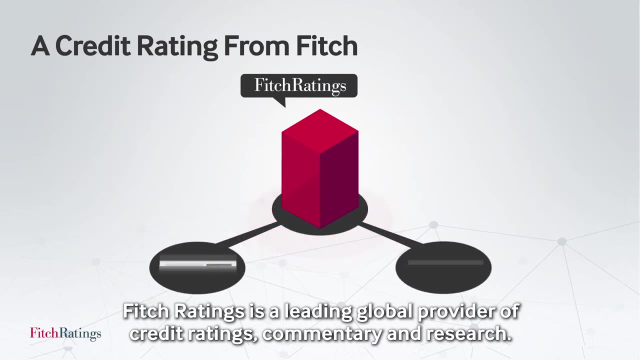 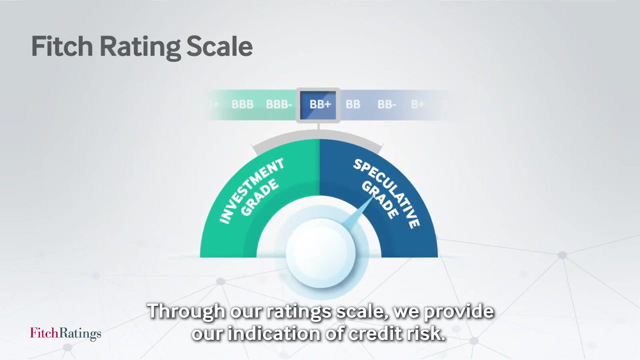 analytical resources. The credit rating is one of these key inputs, and that is how we help investors make important credit judgments on their own with confidence. A credit rating from Fitch. Fitch Ratings is a leading global provider of credit ratings, Credit ratings, commentary and research. Through our rating scale, we provide our indication of 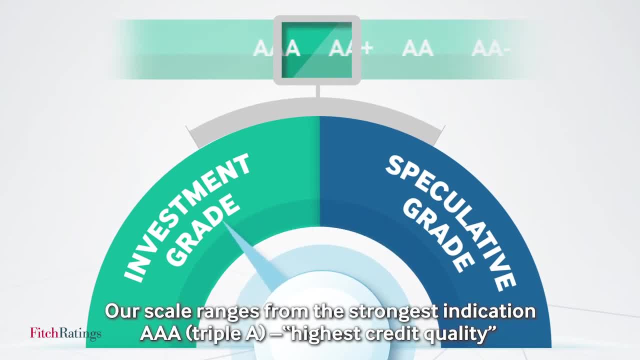 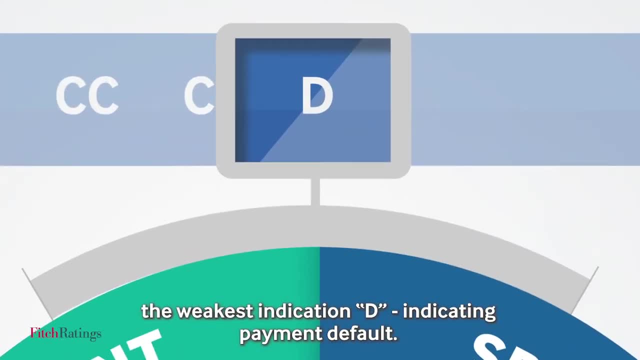 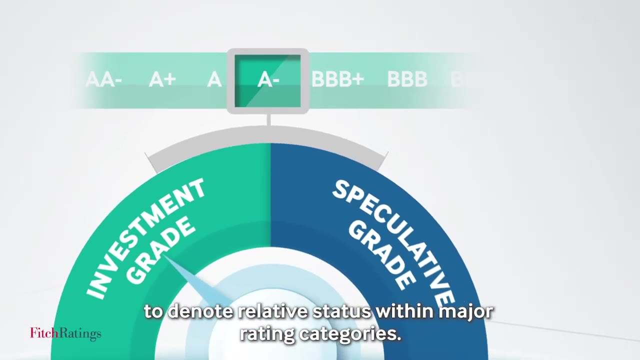 credit risk. Our scale ranges from the strongest indication- AAA- highest credit quality- to the weakest indication D, indicating payment default. The modifier's pluses or minuses may be appended to a rating to denote relative status within major rating categories. We simultaneously assign: 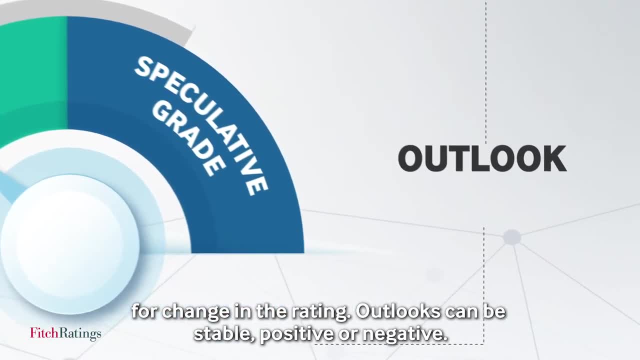 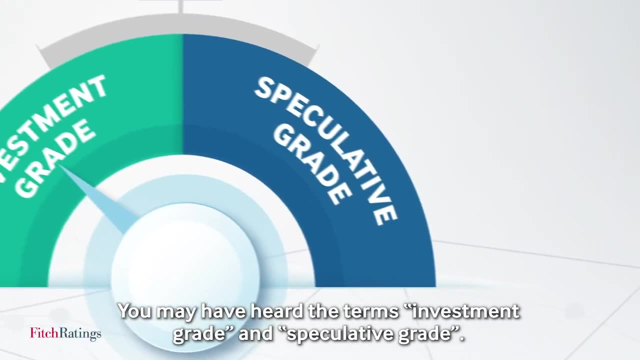 rating outliers to a rating to denote relative status within major rating categories. Outlooks indicating the potential for change in the rating Outlooks can be stable, positive or negative. You may have heard the terms investment grade and speculative grade. This is capital markets. 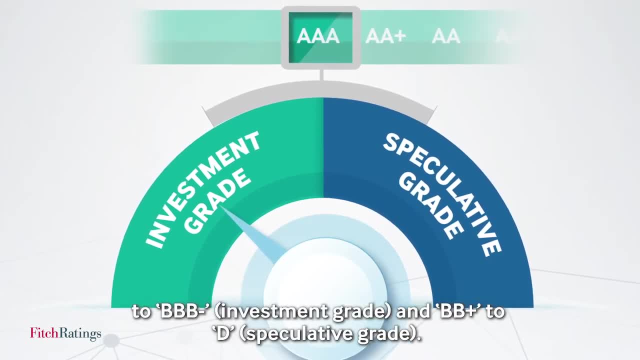 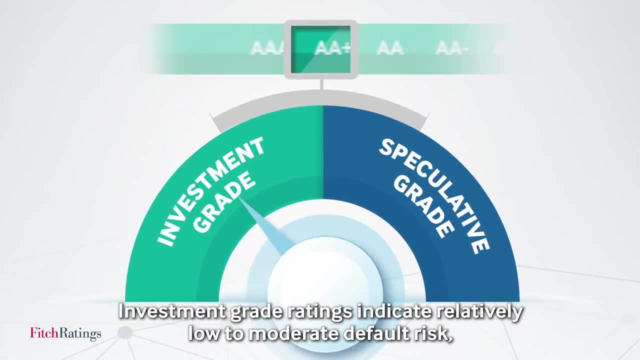 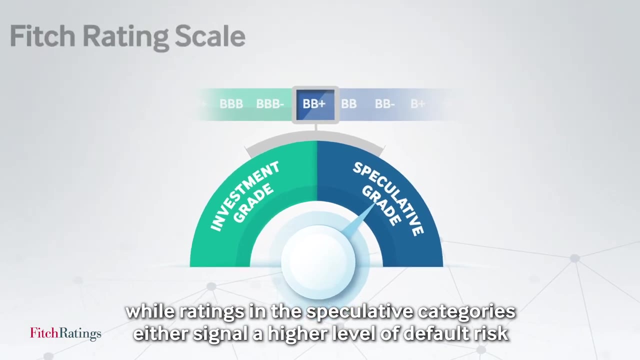 shorthand to describe the categories AAA to BBB- investment grade and BBB- to D or speculative grade. Investment grade ratings indicate relatively low to moderate default risk, while ratings in the speculative categories either signal a higher level of default risk or that a default has already occurred. 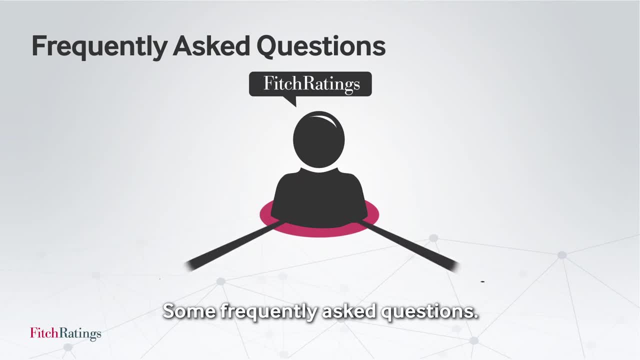 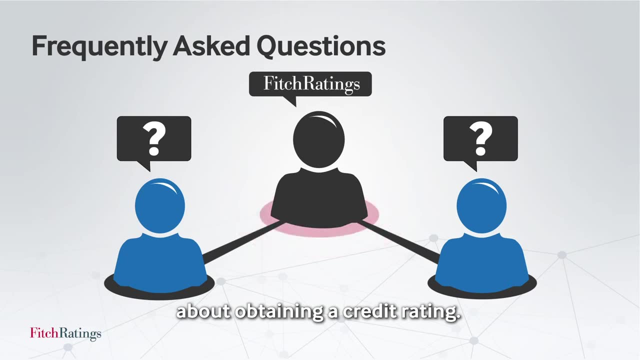 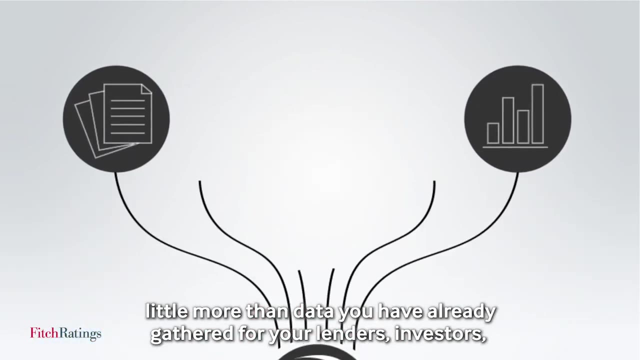 Some Frequently Asked Questions. You may have some basic questions and share common misconceptions about obtaining a credit rating. Gathering the necessary information is straightforward and often requires little more than data you have already gathered for your lenders, investors, regulators or a board of directors. We've heard from 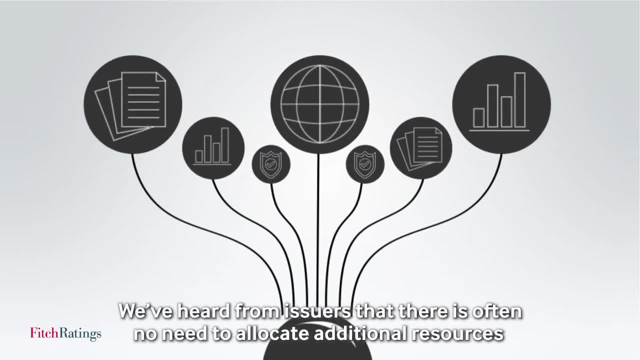 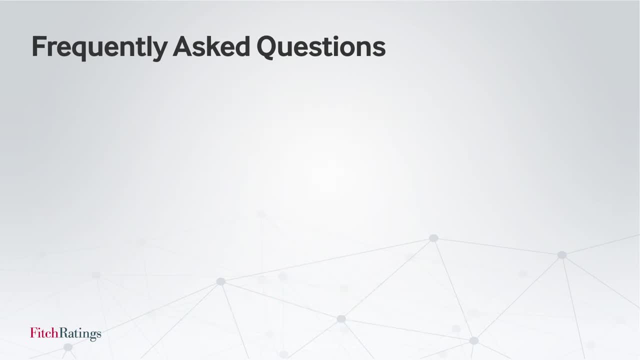 investors, regulators or a board of directors. We've heard from investors, regulators or a board of directors. We've heard from, We've heard from issuers that there is often no need to allocate additional resources or staff to manage the initial process and ongoing maintenance. 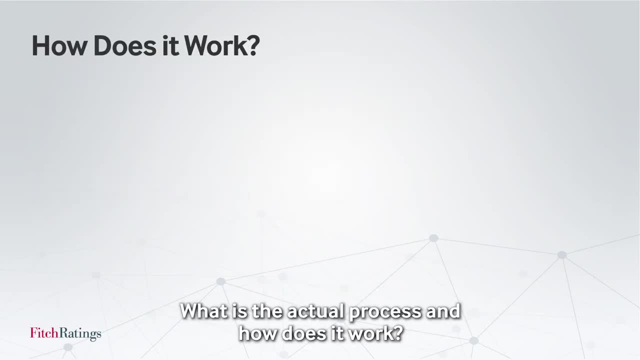 What is the actual process and how does it work? The ratings process typically takes approximately two to four weeks and can vary based on the level of complexity of the analysis. It includes our thorough analysis, independent perspective and transparent methodology. Afterwards we typically provide ongoing surveillance. 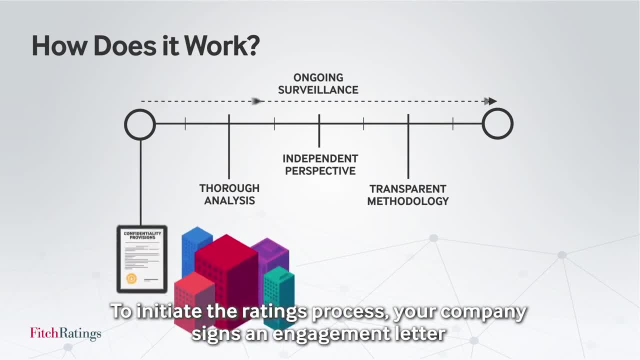 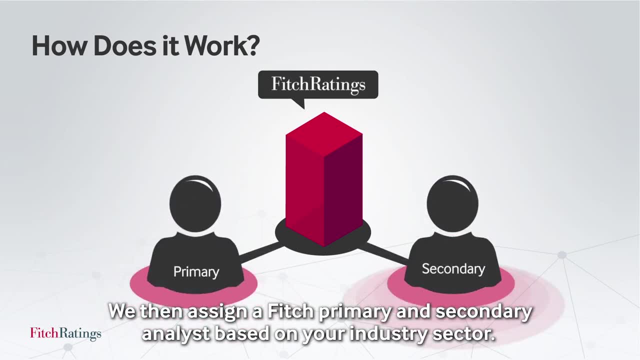 To initiate the ratings process, your company signs an engagement letter which includes confidentiality provisions. We then assign a Fitch primary and secondary analyst based on your industry sector. Our analysts have a wide range of backgrounds and most have worked at financial institutions such as banks, insurance companies, investment houses and financial departments of major 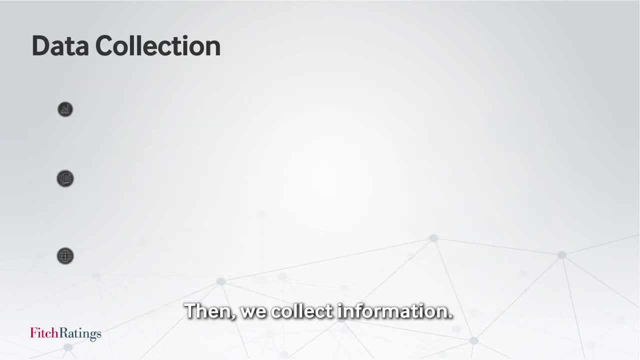 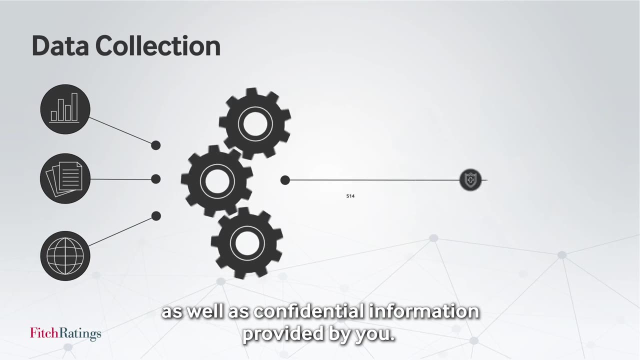 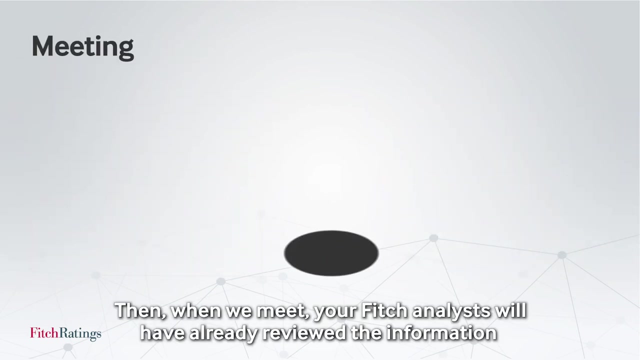 companies. Then we assign a financial analyst, We collect information, We develop our rating rationale based on publicly available information as well as confidential information provided by you. Most companies already have these materials prepared and available. Then, when we meet, your Fitch analysts will have already reviewed the information you. 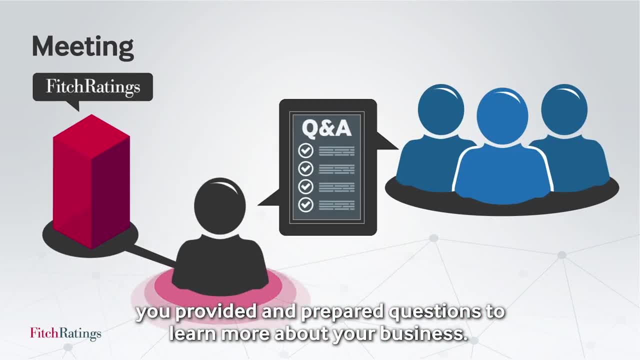 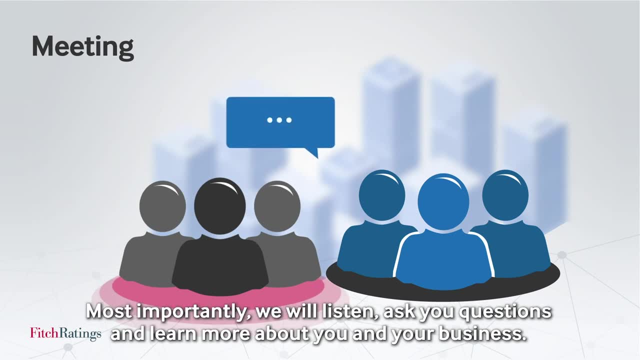 provided and prepared questions to learn more about your business. We will hold a meeting where Fitch analysts will discuss this with you. We will listen, ask you questions and learn more about you and your business. It's also a great opportunity for you to ask questions and have an open dialogue. 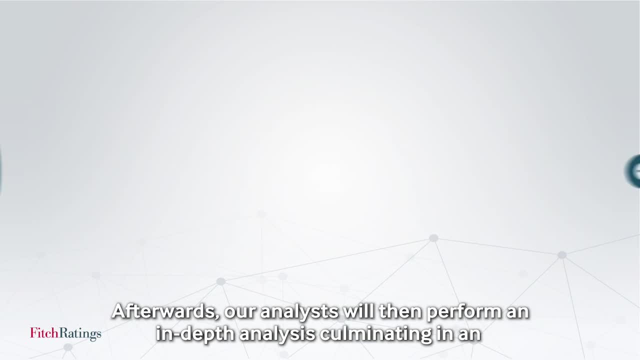 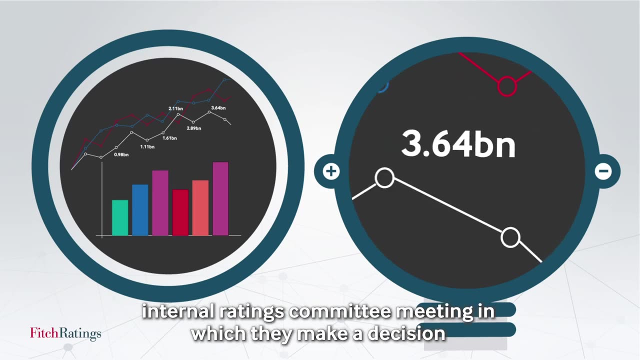 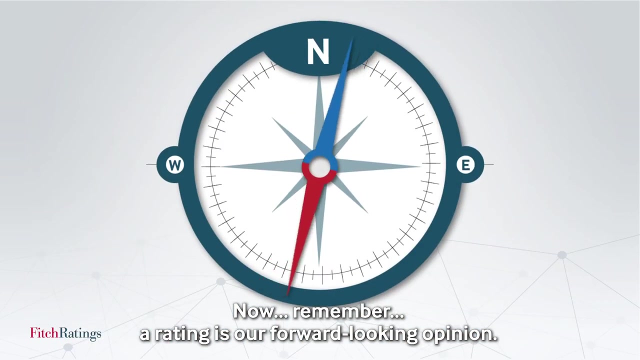 And Fitch analysts will come to you, if you prefer. Afterwards. our analysts will then perform an in-depth analysis, culminating in an internal ratings committee meeting in which they make a decision on the appropriate rating for your company. Now remember, a rating is our forward-looking opinion. 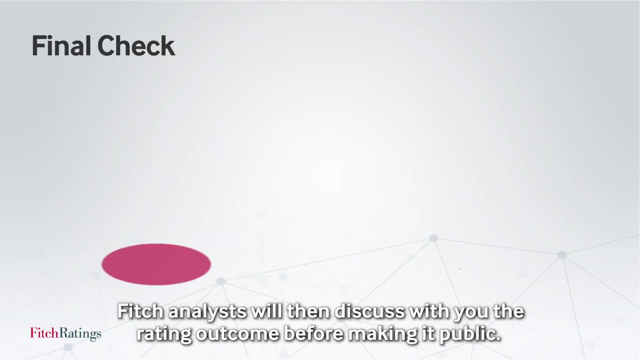 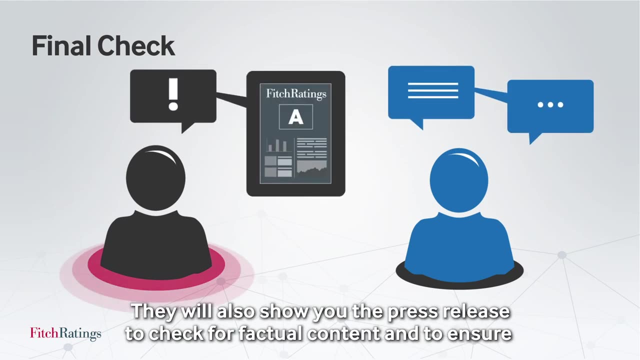 Thank you for watching. Have a great day. Fitch analysts will then discuss with you the rating outcome before making it public. They will also show you the press release to check for factual content and to ensure that any non-public information is not released.